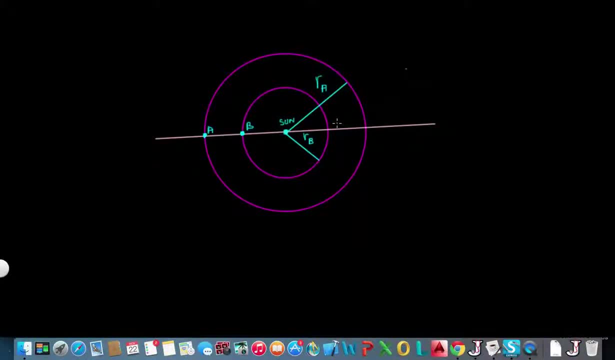 Hello everybody, I'm going to be talking about an interesting astrophysical observation that says that if two planets are in a circular orbit around the sun, that the sine of the maximum angle of deviation, which we denote as theta, is equal to the orbital radius of planet B divided by the orbital radius of planet A. 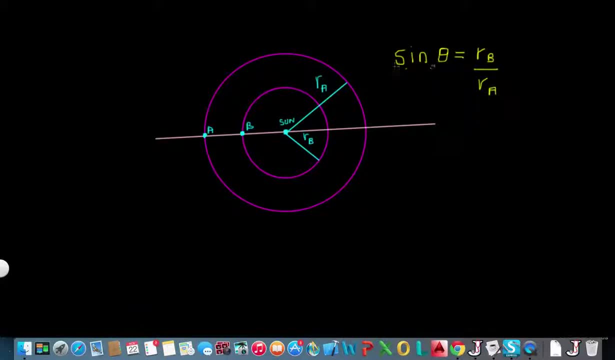 Now this angle. theta is actually the maximum deviation of planet B from the sun in the night sky of planet A. So what this really means is that if I were an observer on planet A and I was gazing at the night sky, I would see something like this: 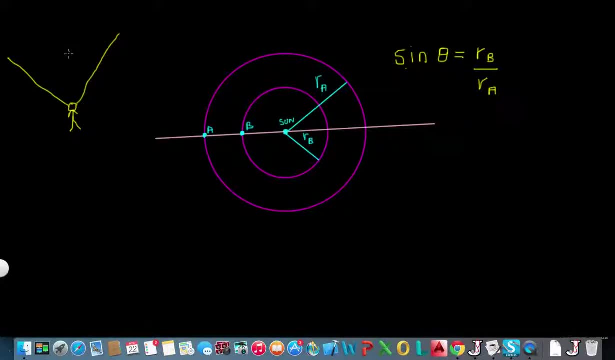 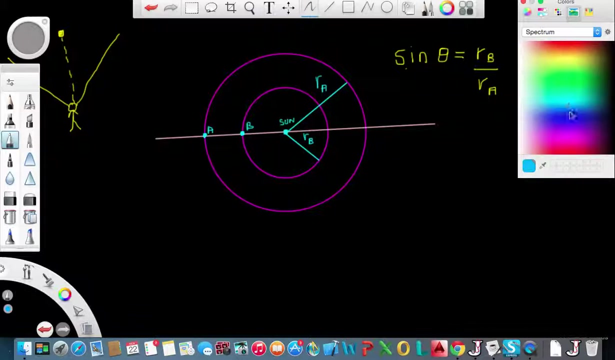 This is my field of vision. So here's my field of vision. So here's the sun, and we're going to call this angle zero And the other planet so planet B would. So I'd see that planet B here. 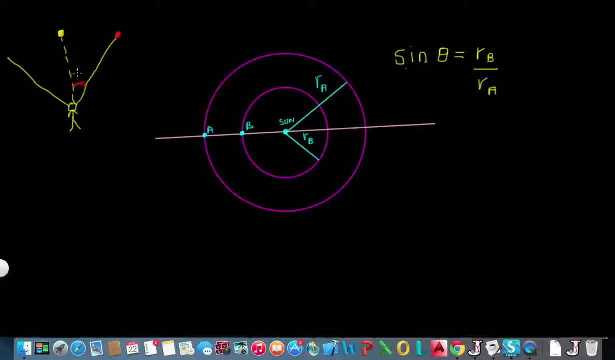 So this is the maximum angle of deviation theta. Now, on this eagle eye view, this angle theta would occur when a tan Tangent is drawn from planet A to the orbit of planet B. Now this is what it's going to look like. 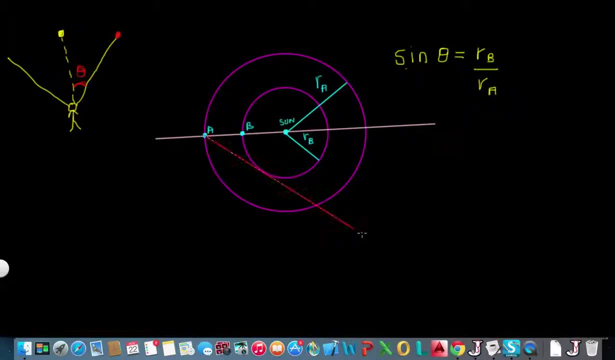 We're going to draw a tangent, And So this point here, this is really just another position of planet B, And whenever planet B is in this position, the maximum angle, The maximum angle of deviation, occurs from the sun, of course. 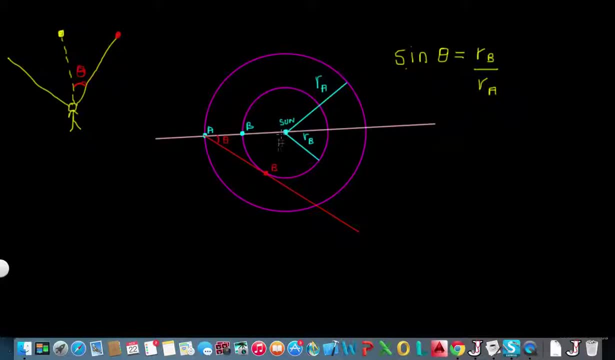 And if you were to drop a perpendicular from the sun, or in other words, the center of the orbit of planet B, you would get a 90-degree angle. So if you were to do that, it would look something like this: And that 90-degree angle.